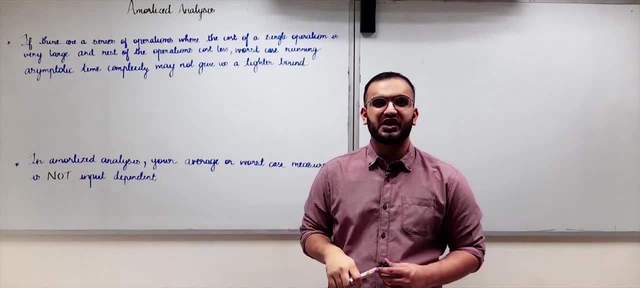 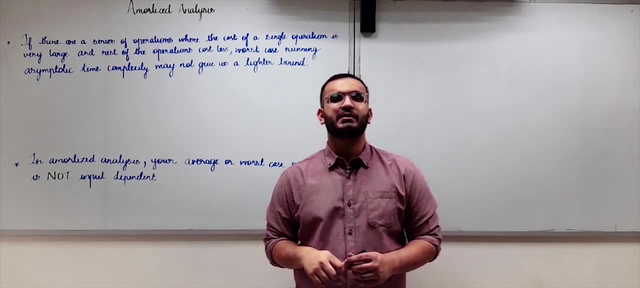 Hi friends, welcome to my channel. So this is the first topic of advanced data structures playlist, amortized analysis or amortized time complexity. So you would have already heard about asymptotic time complexity and how it is used to calculate the time complexity of different operations. 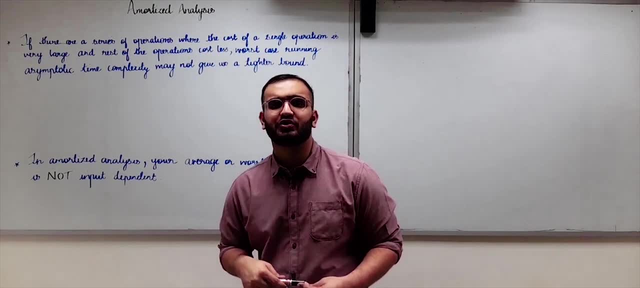 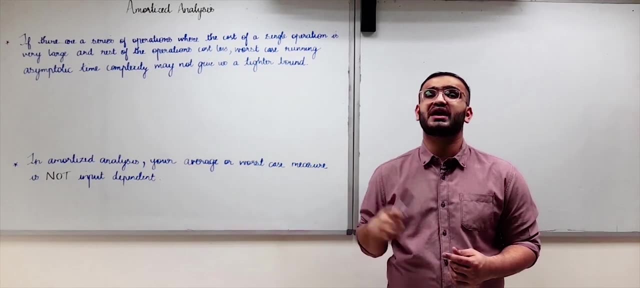 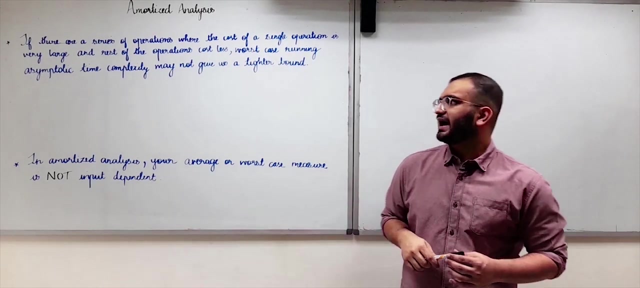 and in that you would have also heard about, about big O notation, the theta notation and all that. So in this video we are going to talk about why amortized analysis or amortized time complexity computation is more important than asymptotic time complexity computation in some cases, And I will also give you a very simple explanation with the help of an 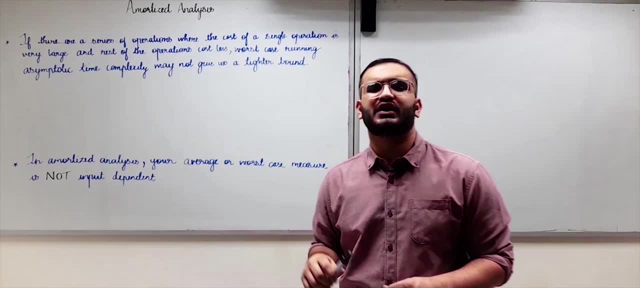 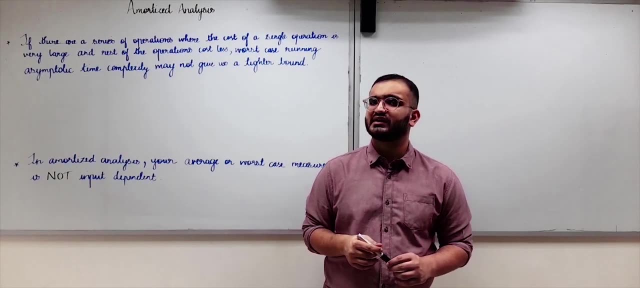 example. Then we will talk about a very important feature of amortized analysis and I will finally end this video with the help of an example of augmented stack and how amortized analysis is helpful when we are doing time complexity computation for augmented stack. So first, 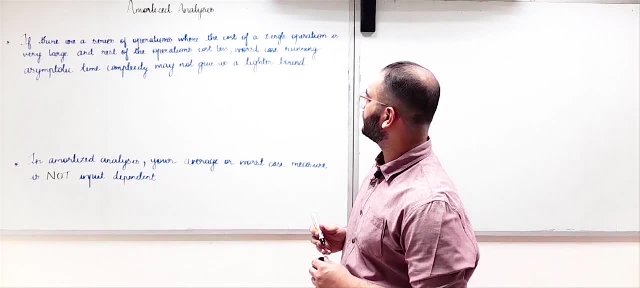 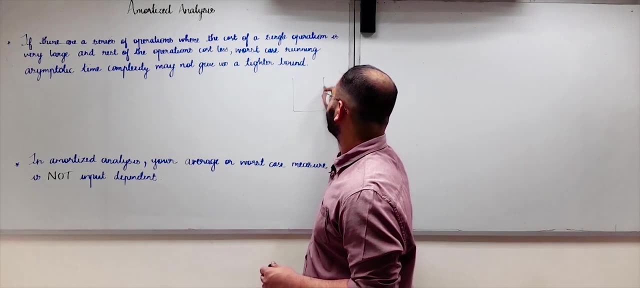 of all I have written over here- if there are a series of amortized time complexity operations where the cost of a single operation is very large. So let us consider a data structure. It can be any data structure, So in that many operations are performed, There are many operations. 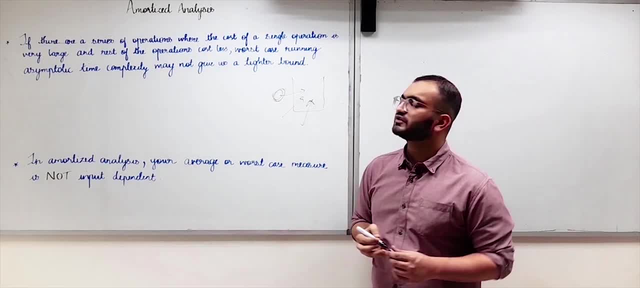 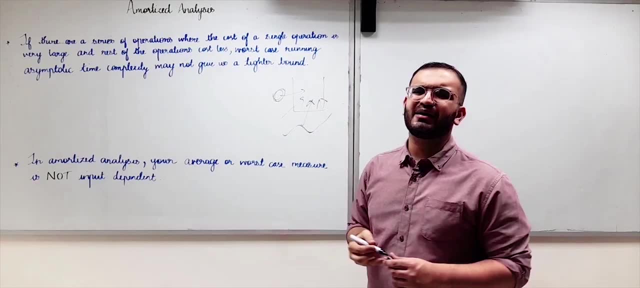 But there is this one single operation: Time. complexity of this operation is very large, or the cost of this operation is very large, While the rest of the operations, while the rest of the operations, the cost of these rest of the operations, is less So in such 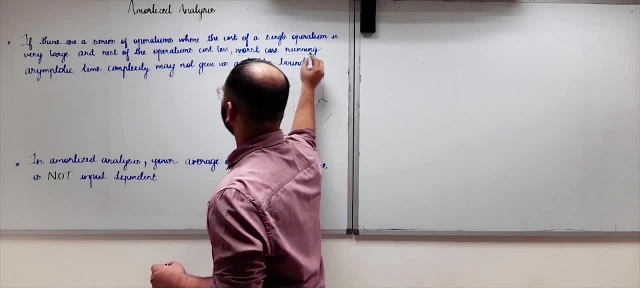 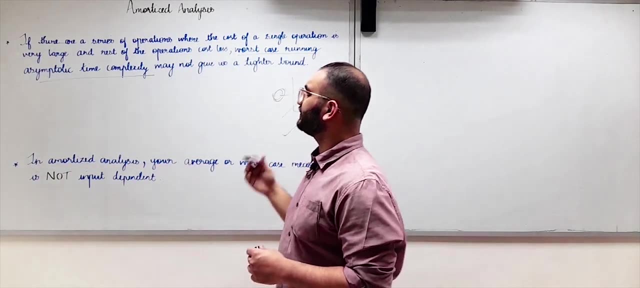 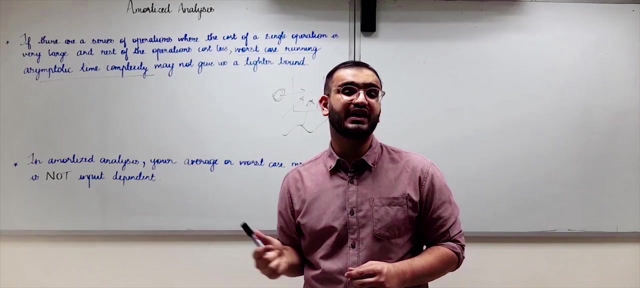 case, The worst case, the worst case- running asymptotic time complexity may not give us a tighter bound. Now, what this means is that, in such cases, what we actually do in case of asymptotic time complexity computation, is that we find out the operation with the worst case: time. 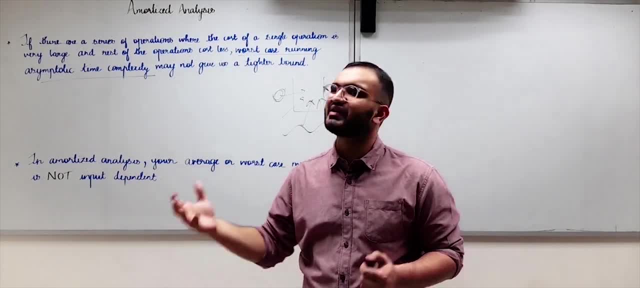 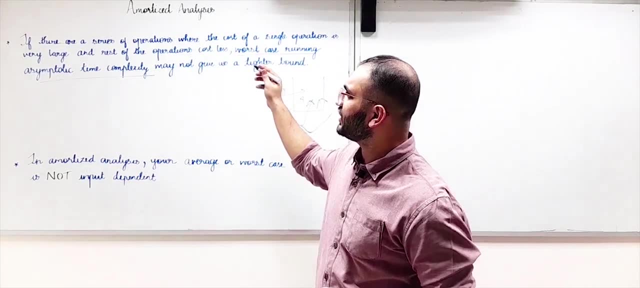 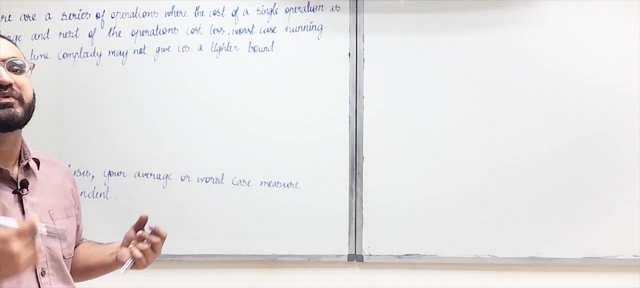 complexity, and then we multiply it with the number of operations, And this is how we get the time complexity for the total number of operations right. This is how we do it, But in such cases this is not a useful method. So now let us discuss a real life example where amortized analysis is a better option. 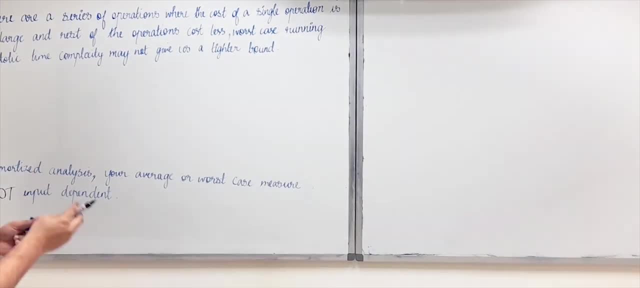 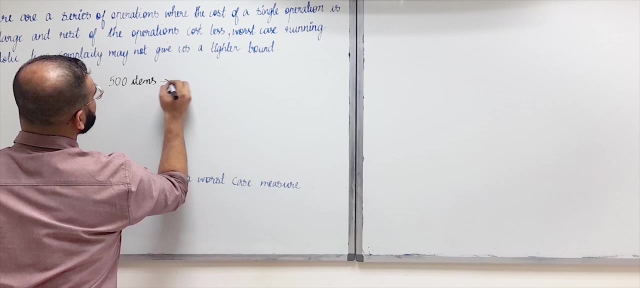 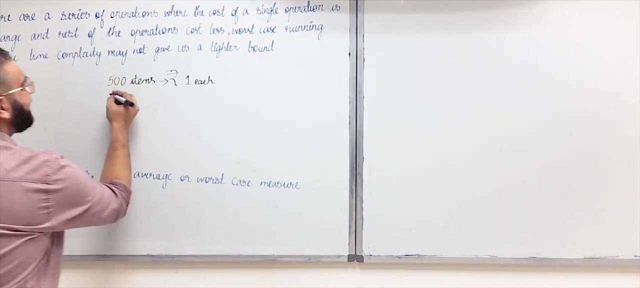 than asymptotic analysis. Suppose there is a shop in which there are 500 items, okay, And the cost of each of these items is rupees 1, right, Each of these items costing rupees 1, right. And there is another item in the shop- You can call it the 500- and one item. 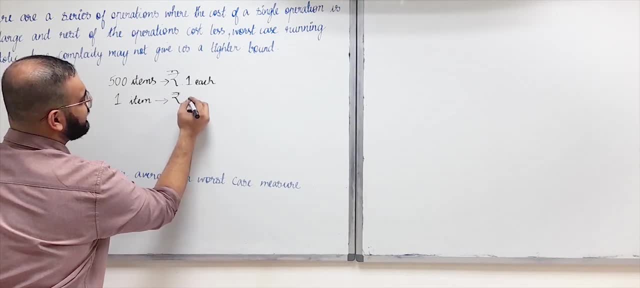 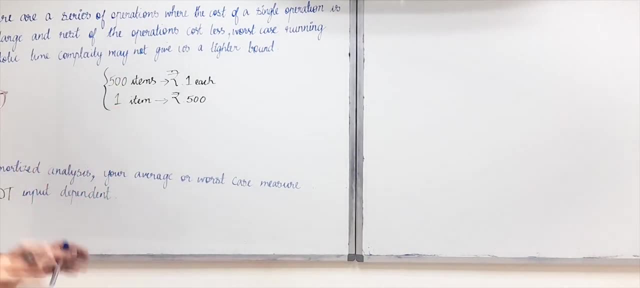 right, the cost of this item is very large. it the cost of this item is rupees 500. okay, so in total there are 501 items in the shop. okay, suppose I want to buy all these 501 items from this shop. okay, and I don't know how much money should I? 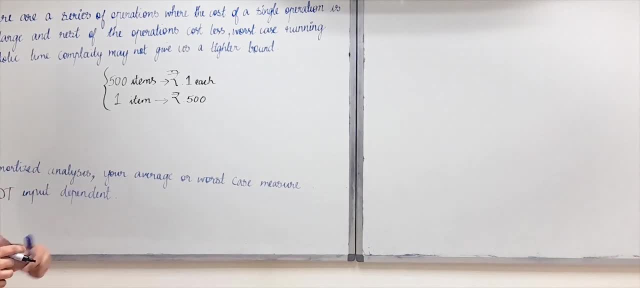 take with myself in the shop in order to buy all these 501 items. so I asked my friend Asim and Aman to tell me that how much money should I take with myself in the shop so that I can buy all these 501 items? so when I asked Asim, as he is a 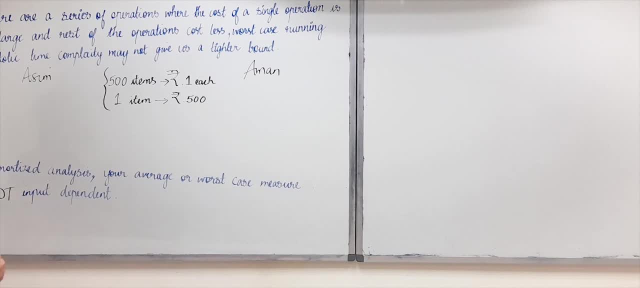 very conservative guy and he always wants to be on the safer side. so what he tells me is that the maximum price of any item in the shop is rupees 500. okay, this is the item with the maximum price. so you should take 500, the maximum price of any item in the shop, into the number of items in the 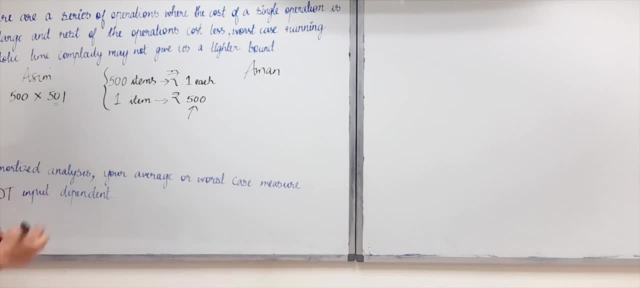 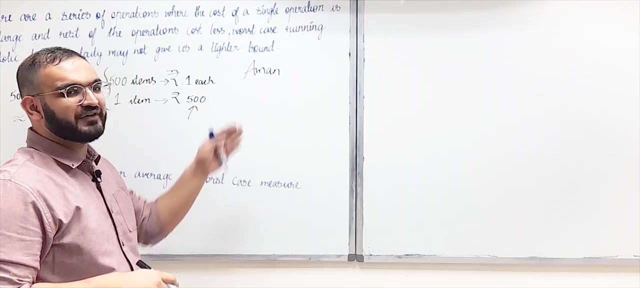 shop into the number of items in the shop, that is 501, right, so he? so he's asking me to approximately take two lakh fifty thousand rupees when I visit this shop to buy all the 501 items. okay, and now there is another friend of mine that. 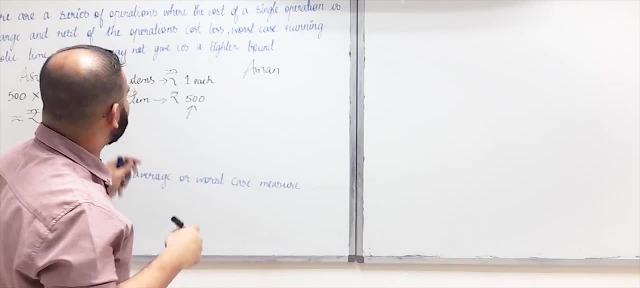 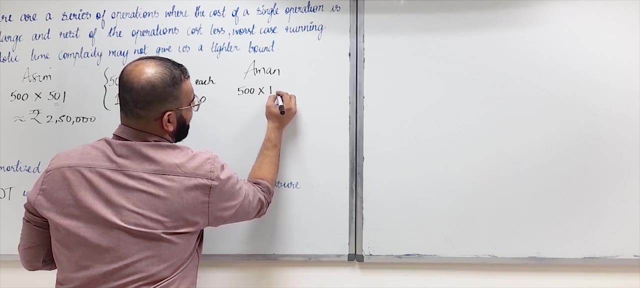 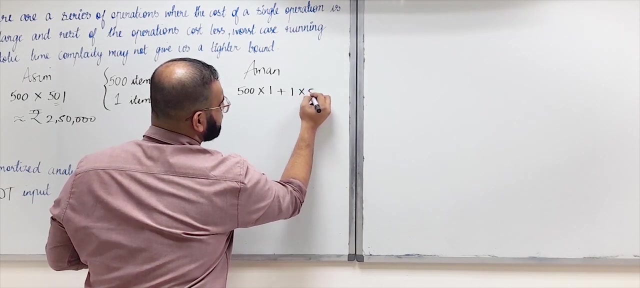 is Aman. he makes his own calculation and he says: okay, there are 500 items with rupees one each. five hundred into one, plus there is one single item whose cost is 500. okay, one item whose cost is 500, so you take thousand rupees with you. 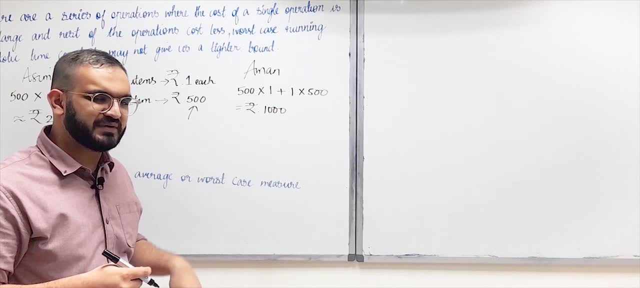 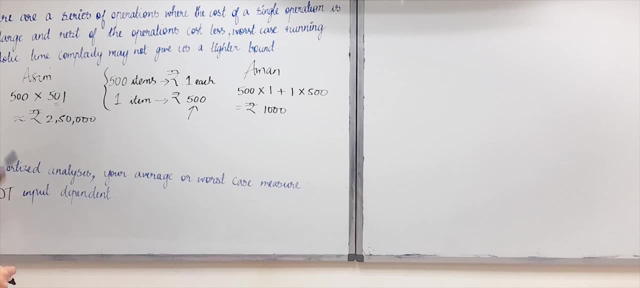 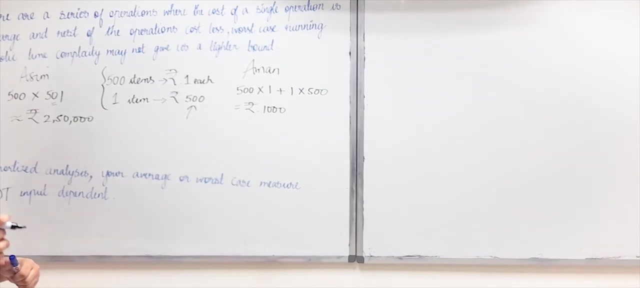 in the shop. so he tells me to take thousand rupees with me in the shop so that I can buy all these 501 items. so now, whom should I listen to? should I listen to Asim or should I listen to Aman? of course I should listen to Aman. why? because Aman is doing a better analysis. 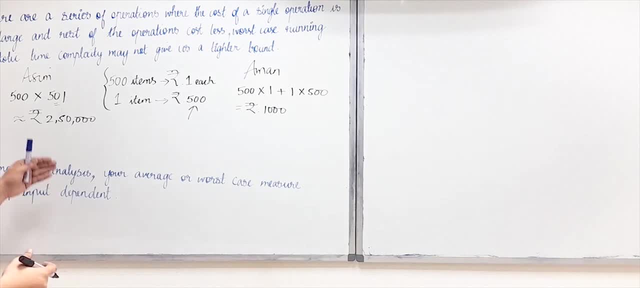 of the cost. then Asim, right, Asim over here is just focusing on the item with the maximum price and on the basis of that he is multiplying it with the total number of items and he is doing his calculation right. so he's kind of doing a worst-case analysis, right, whereas Aman over here is giving a much accurate or a 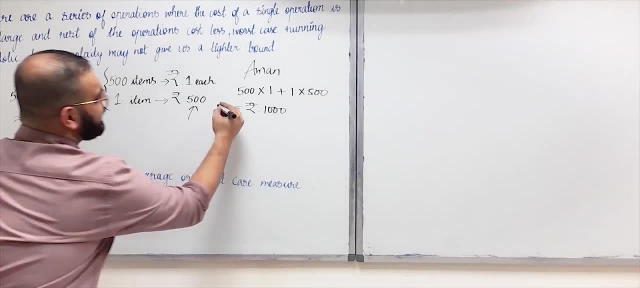 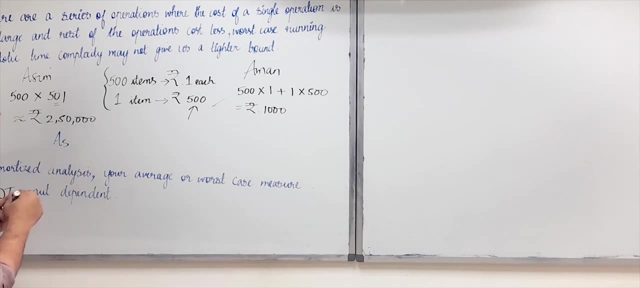 better analysis than Asim, so I would definitely go with aman. so, if you have not noticed until now, Asim over here is the asymptotic analysis, right? Asim over here is the asymptotic time, complexity computation or the asymptotic analysis, whereas aman is the gamut. 처� Alma isين. 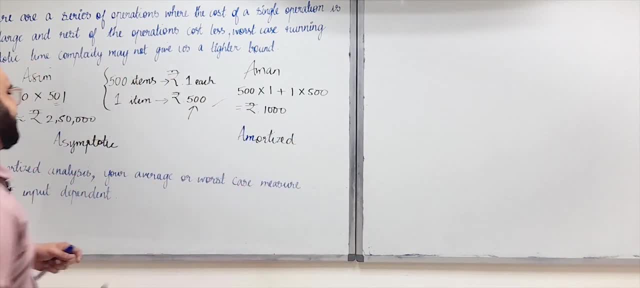 Amman, is the Ammortized analysis right. so what I mean by this is that he is Imagining that there is an actual cost per probability which isВот as candle, on which you have a 10000 units here, which is 1.50, you are going to lose all your loot time. so after the total amount, you just need to charge 3 reaches ofUP to get the amount after being called down and we go to showing us ID to säорmb opera, which is Six units and photos I am never showing, showing you how the life spoke uniqueness, but what I say. I peel some points, but what I don't know how. 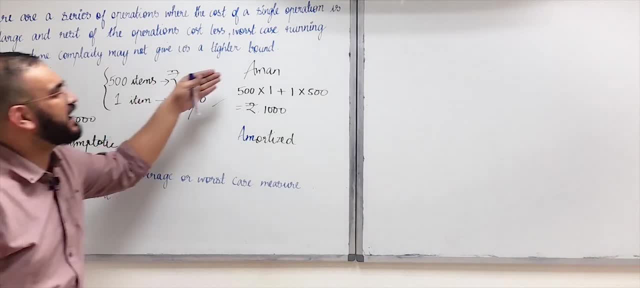 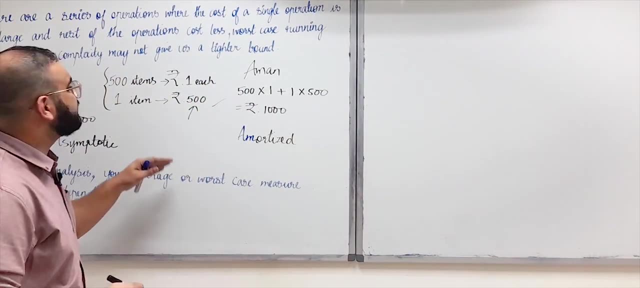 Aasim is doing is an asymptotic analysis, whereas Aman believes in amortized analysis. that is why he is giving us a more accurate analysis in such a case where in the shop, just one single item has a very large price as compared to the rest of the items which have a lower price right. so in such a case, Aman's 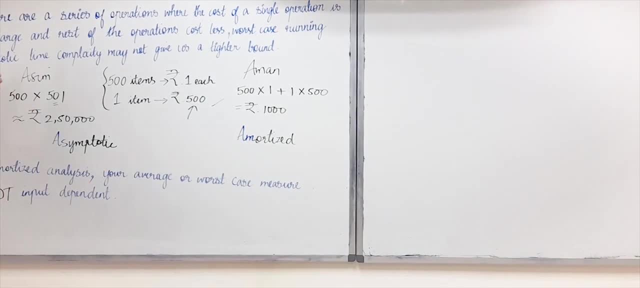 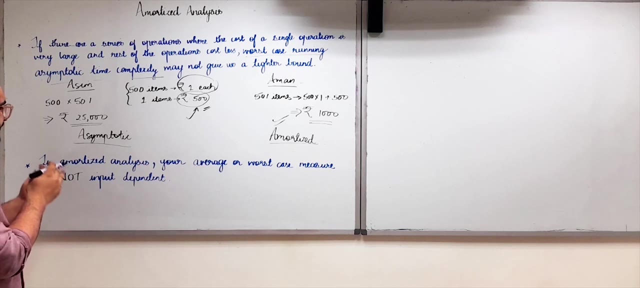 analysis, or the amortized analysis, is a better option than Aasim's analysis or the asymptotic analysis. now let us look at a very important feature of amortized analysis, which is that in amortized analysis, your average or worst-case measure is not input dependent. so what this means is that, as you would have, 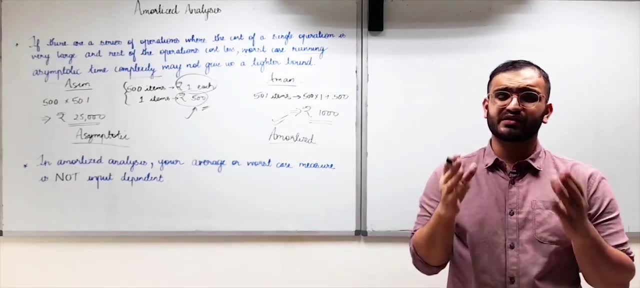 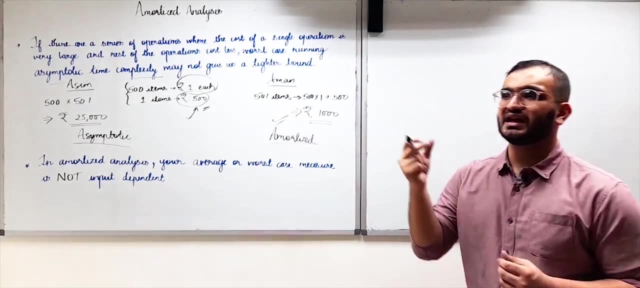 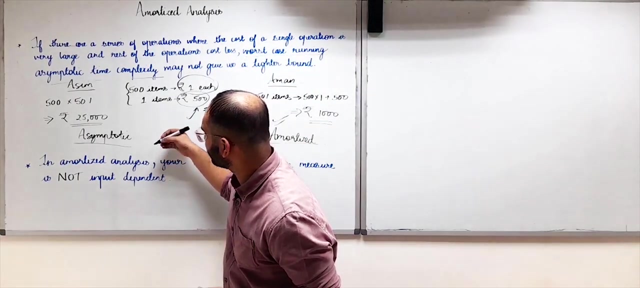 seen. in case of like quicksort, we say that the asymptotic worst-case time complexity. when the input is sorted, we say it is big of n square, right, so this when the input is sorted, all these things that are input dependent, they are not really important in case of amortized analysis. let us look at 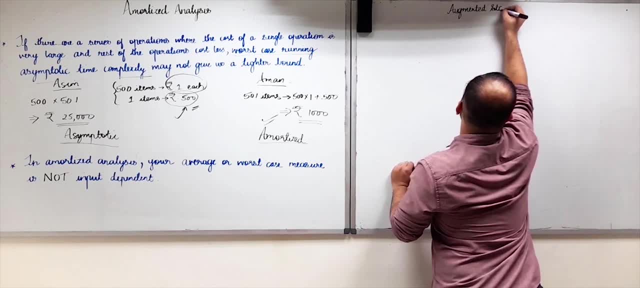 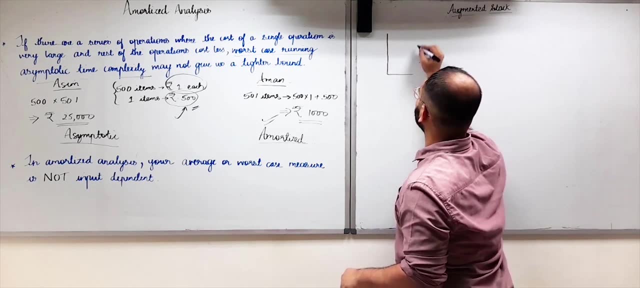 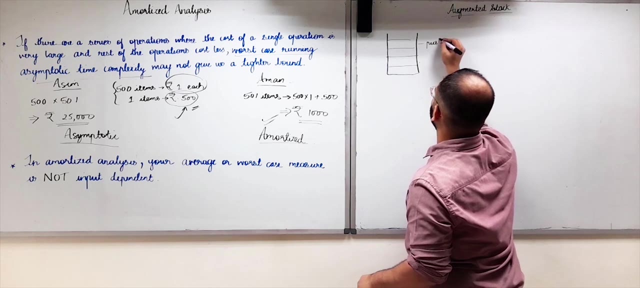 augmented stack. now, first of all, let me tell you what is augmented stack. we will learn augmented data structures later on in this playlist, but you might already be knowing the normal stack, which has basically two operations. the first one is push the time complexity of which is order of one, and pop the time complexity. 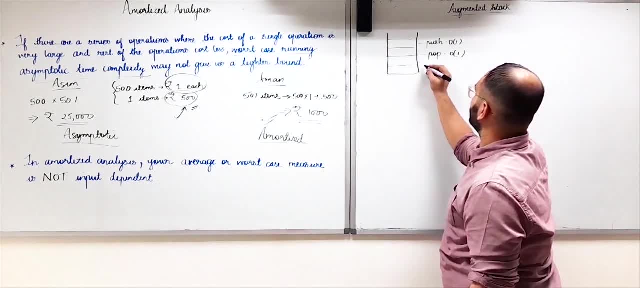 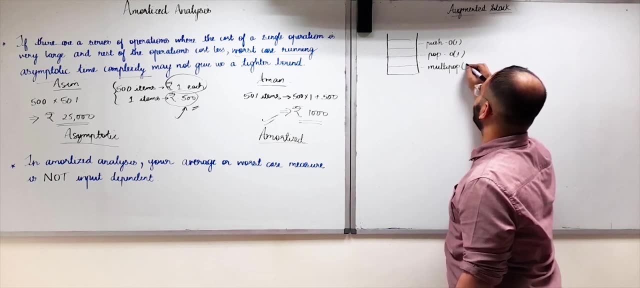 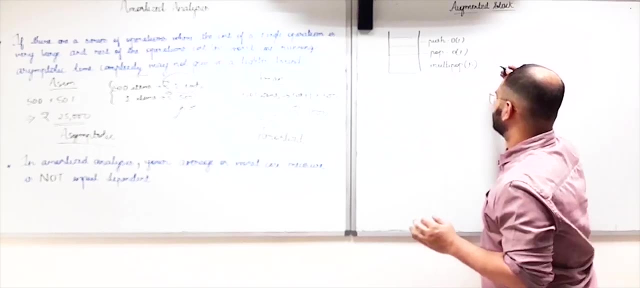 of which is again order of one right. so now let us consider another operation in this augmented stack, which is multipop of K, where K is the number of elements that we want to pop out at a single time out of this stack. right, and this multipop of K is actually defined something like: 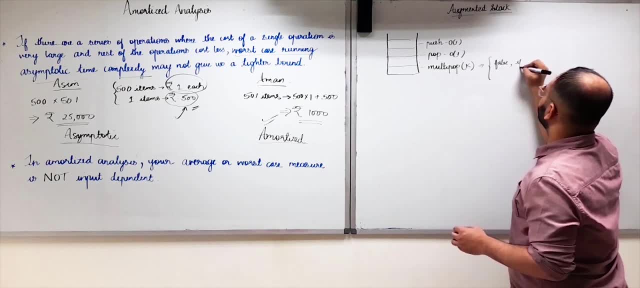 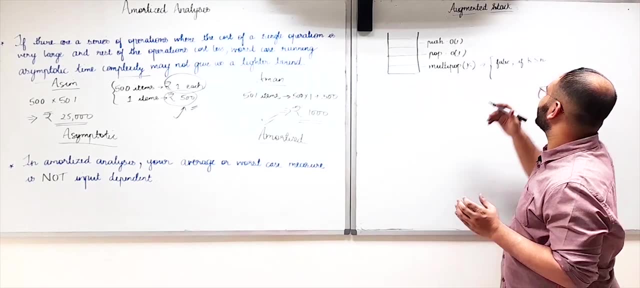 this, that it returns a false if K is greater than n. of course, when I want to pop out the number of elements from the stack that are greater than the number of elements already present in the stack, that's not possible. So that is when it will return. 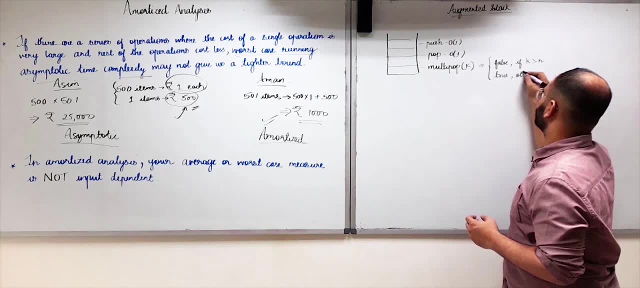 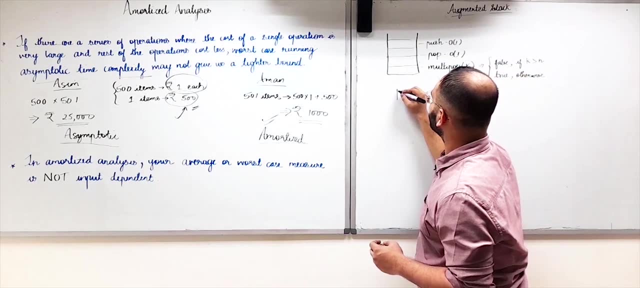 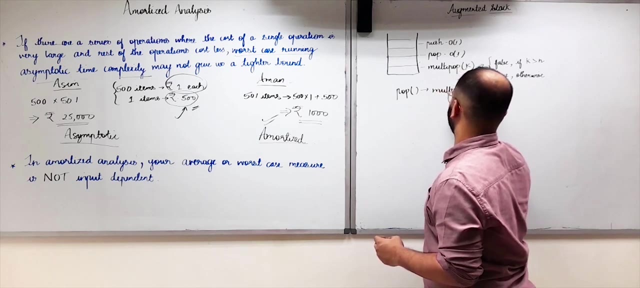 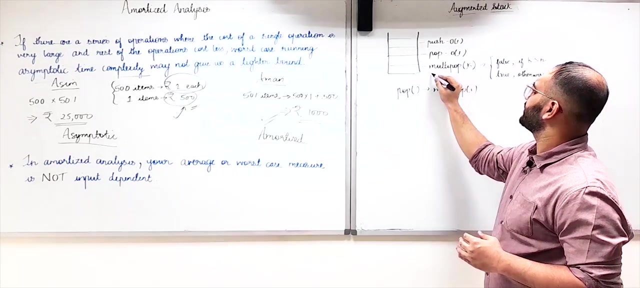 false and it will return true otherwise. So this is my multipop of k. Now you can also consider the pop operation as multipop of 1.. Easy to understand. So now, what can be the worst case? time. complexity of multipop of k. We found out the time. complexity of. 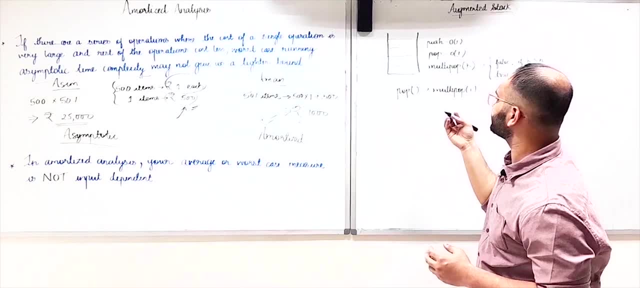 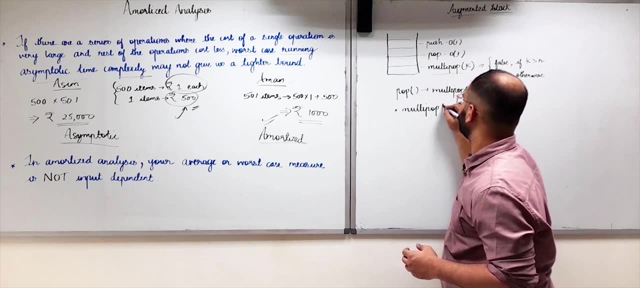 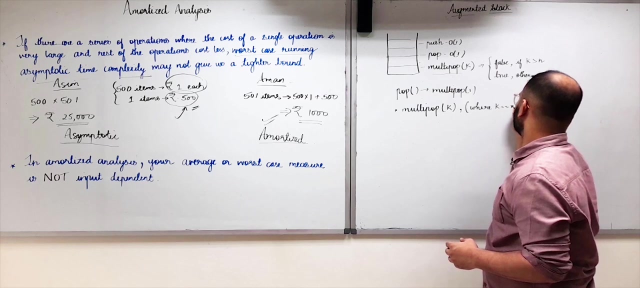 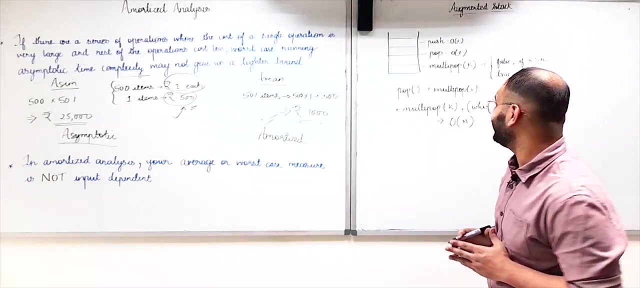 push and pop. What about the time complexity of multipop of k? Of course, if we are asked to find out, if we are asked to perform the operation multipop of k where k is equal to equal to n. in this case, the time complexity of multipop of k will be order of n, right? 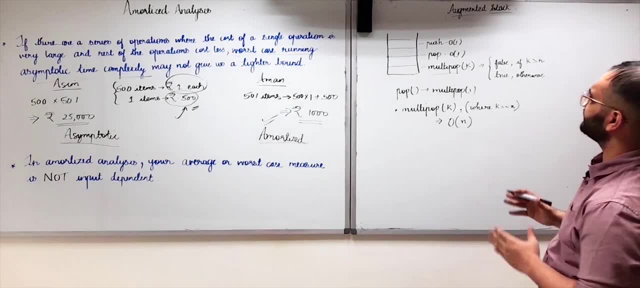 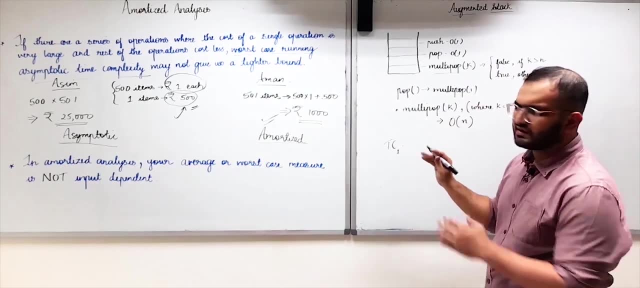 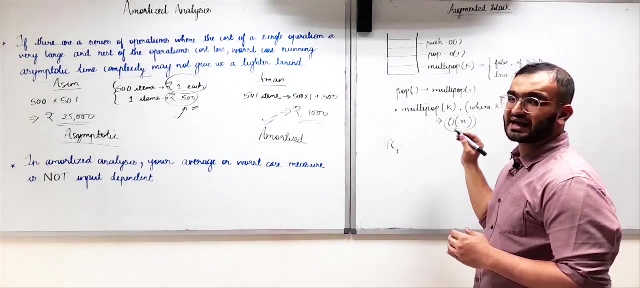 So now, if suppose we want to do the time complexity analysis of this data structure, which is augmented stack, what we will do is that let us name this as time complexity analysis. 1. We will see, okay, the operation with the worst case: time complexity, the time complexity. 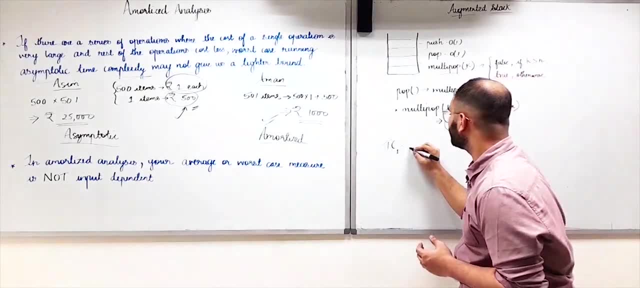 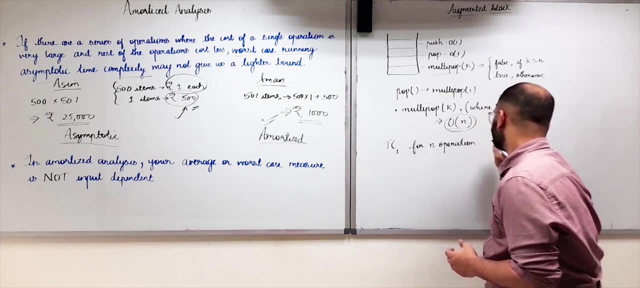 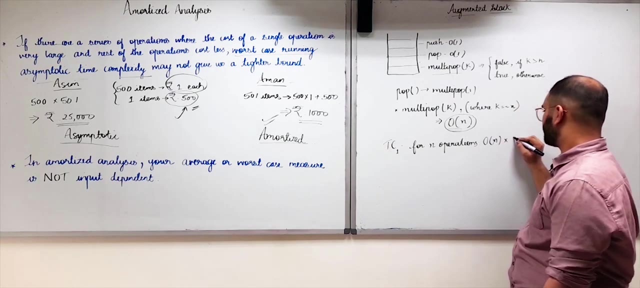 of that operation is order of n, And suppose we are doing it for n operations, right? So the time complexity for these n operations will be order of n into the number of operations, that is n. So the time complexity for these 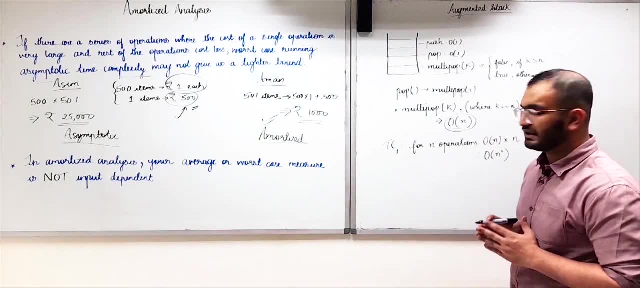 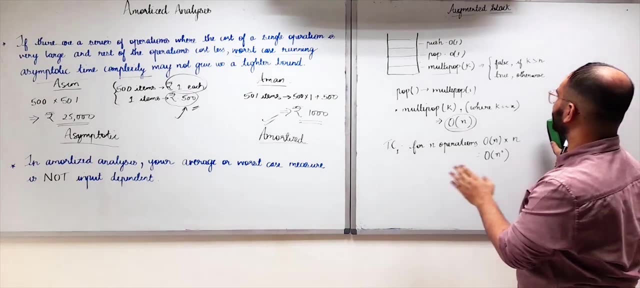 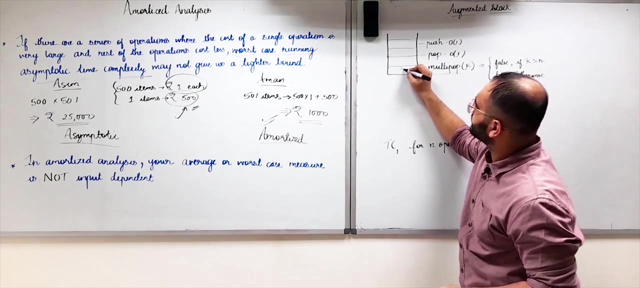 n operations will be order of n square, right. So this is how we are going to do it. But there is a catch in this, So we found out. okay, the time complexity should be order of n square. But just consider one thing. that suppose there were 3,, 2,, 6, 9.. Suppose these. 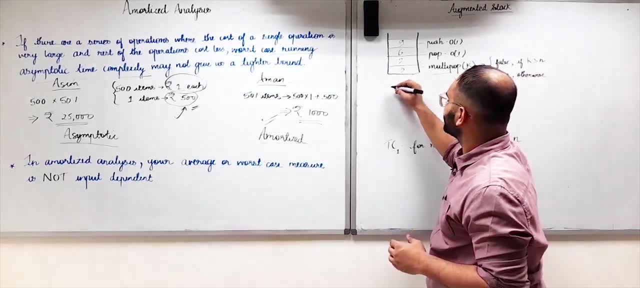 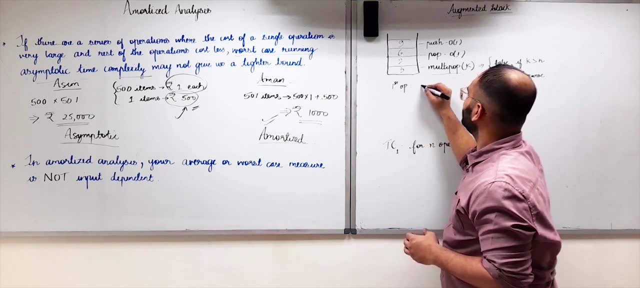 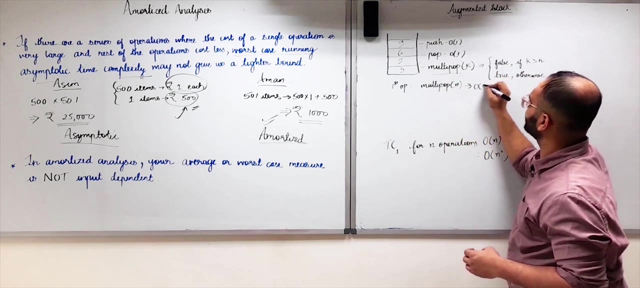 were the elements in our stack, in our augmented stack. And again we try to do the time complexity analysis And the first operation that we perform is multipop of n, right, So now, as already mentioned, the time complexity of this is order of n. Then the second operation. 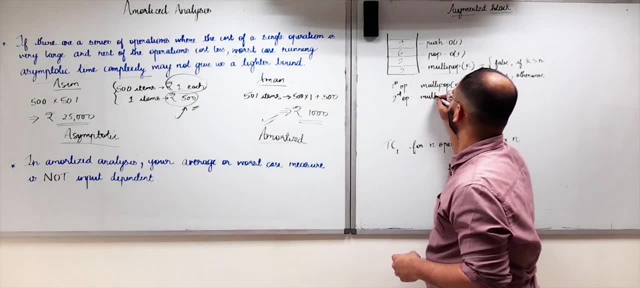 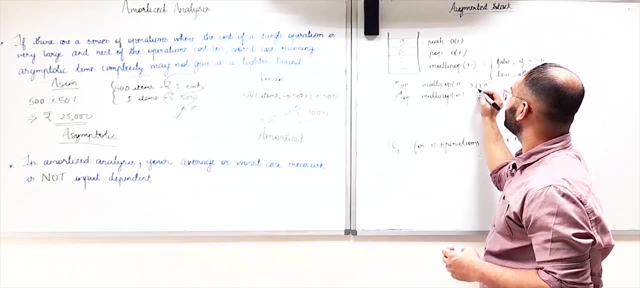 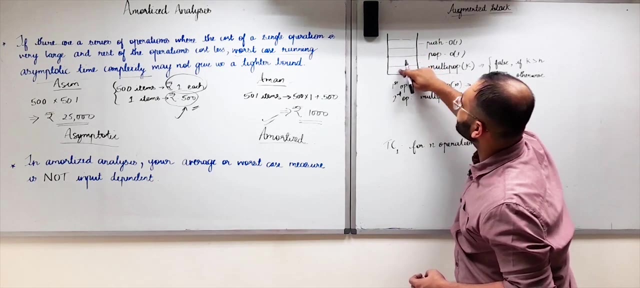 that we perform is multipop of n. Is this possible? No, This is not possible. This is not possible Because when we perform multipop of n, what we actually did was we popped out all the elements. So in the next step or in the next operation, again, it is not possible. 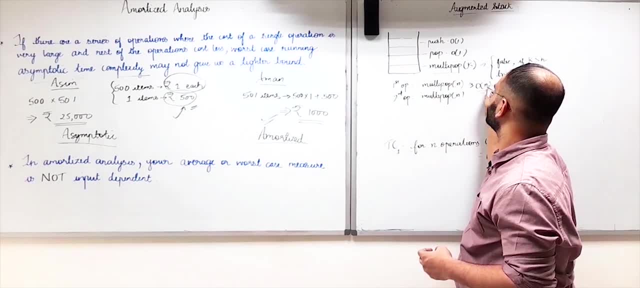 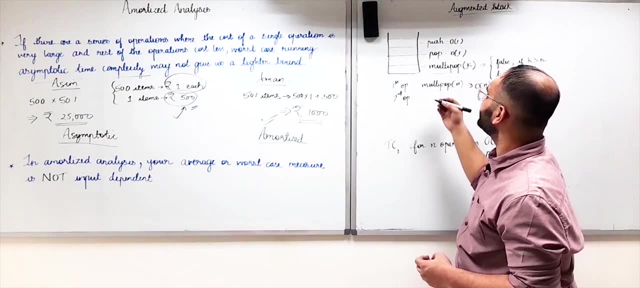 to perform this operation- multipop of n- with a time complexity of order of n. So, again, to perform multipop of n. actually, what we need to do, we need to push in those number of elements again Right, So I don't remember the elements- but we need to do another operation, Which is to 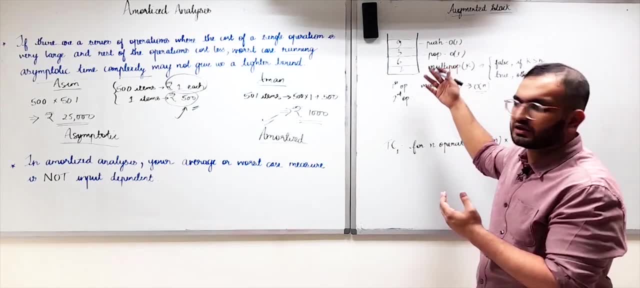 perform telesilo. This time complexity of n factor will raise the next step, or this all number of elements will raise. By doing that, we are actually managing the deciding push in the elements back. so for that, what we need to do for the next n. 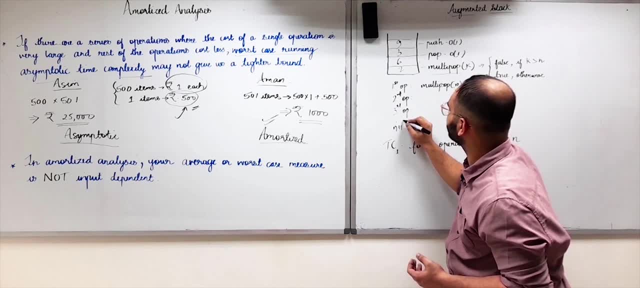 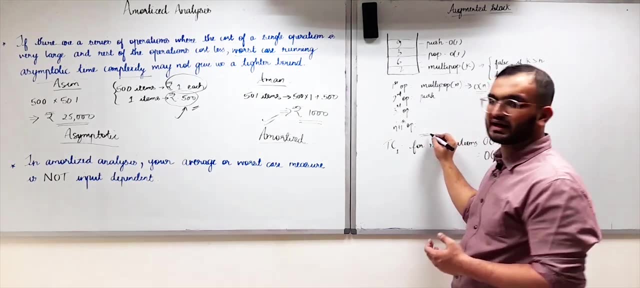 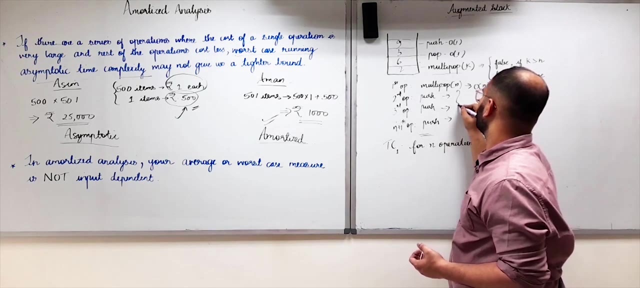 operations till the n plus 1th operation. we need to perform just push. if we need to perform this multipop of n again over here, right, we just need to perform push and, as you know, the time complexity of push is always order of 1. so what we did over here, now again, if we 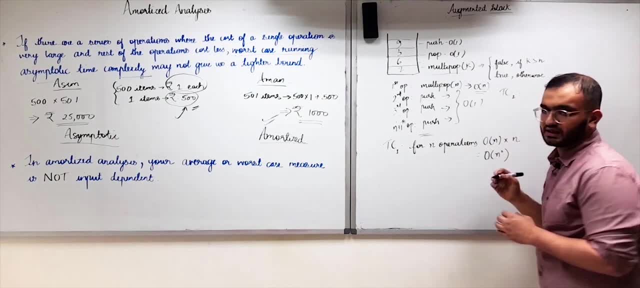 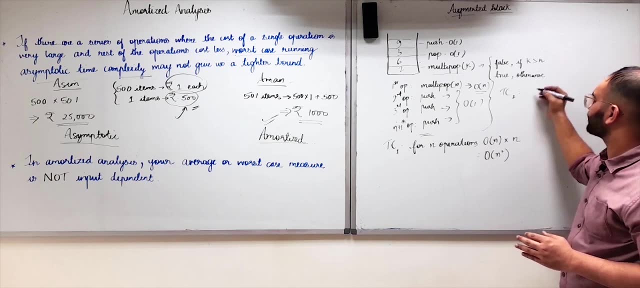 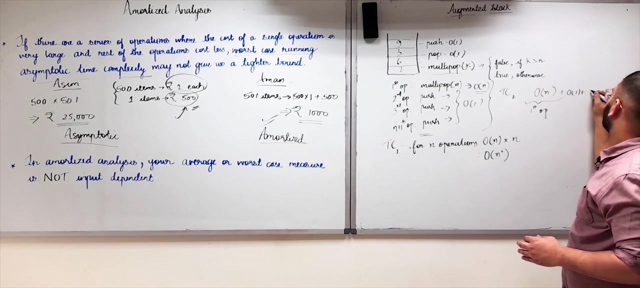 do the time complexity analysis. let's call this time complexity analysis. 2, actually our total time complexity. for all these n plus 1 operations, the total time complexity is basically order of n- this was for our first operation, right- plus order of 1- how many times this is? 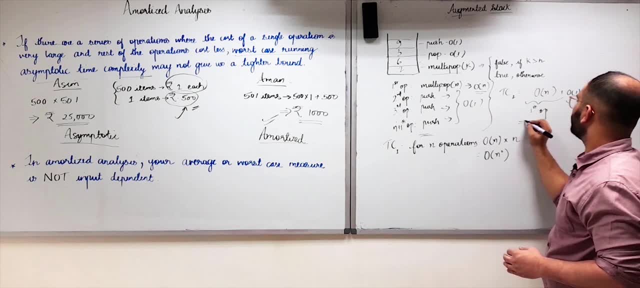 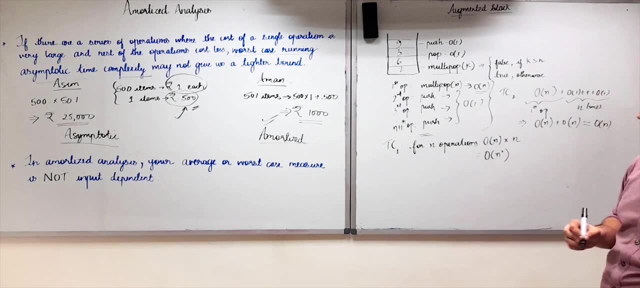 n times. so this is basically order of n plus order of n, or you can call it order of n, but here we found out that time complexity analysis was order of n? square, and whereas here we found out that it was order of n. so this was basically our asymptotic analysis, or the